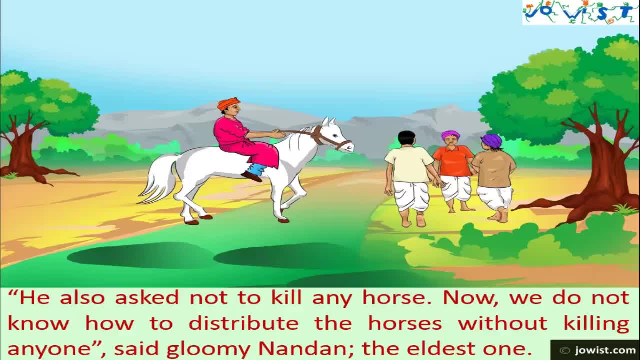 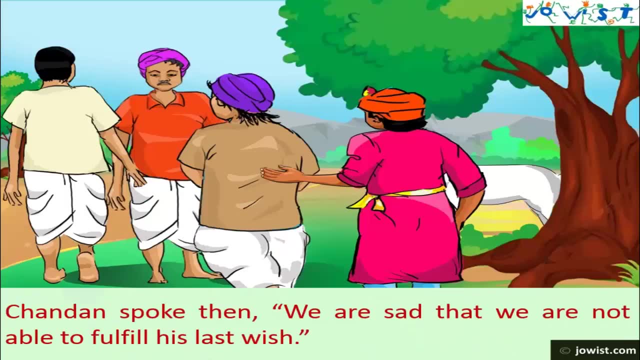 We do not know how to kill any horse. We do not know how to kill any horse. distribute the horses without killing anyone", said the gloomy Nandan. the eldest one, Chandan, spoke then. We are sad that we are not able to fulfil his last wish. 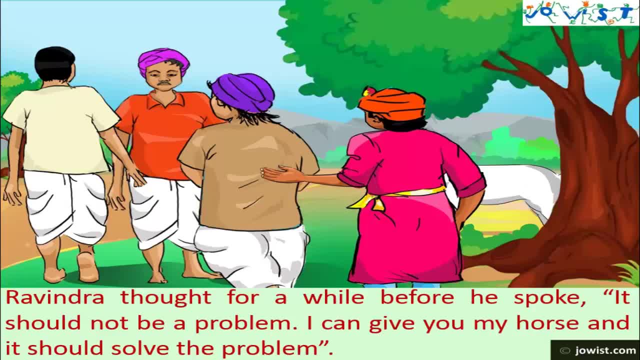 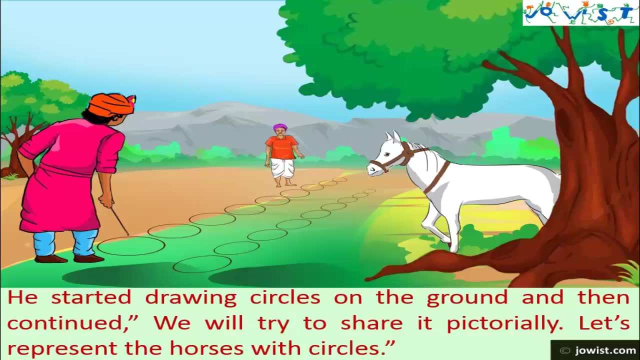 Ravindra thought for a while before he spoke. It should not be a problem, I can give you my horse and it should solve the problem. He started drawing circles on the ground and then continued: We will try to share it pictorially. Let's represent the horses with circles. 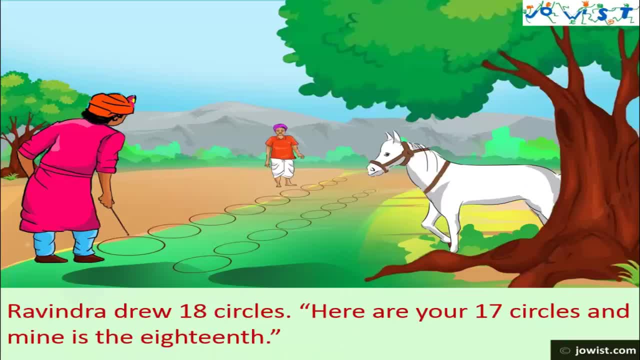 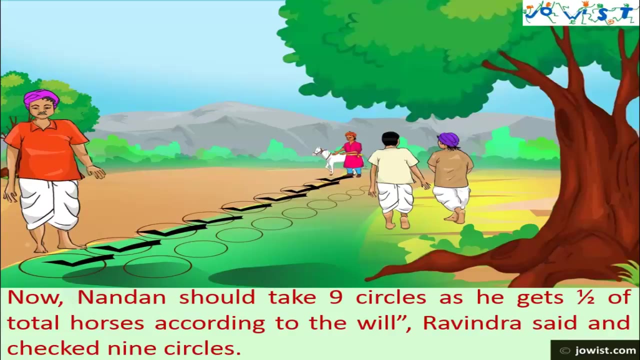 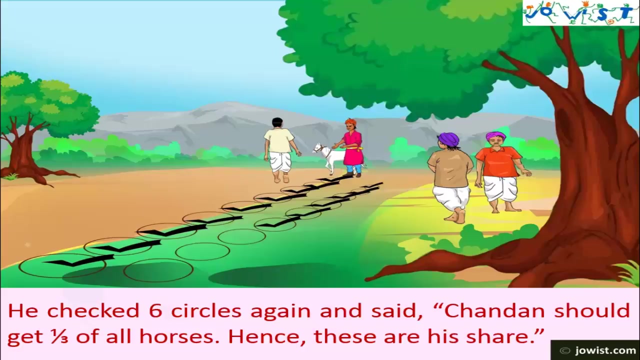 Ravindra drew eighteen circles. Here are your seventeen circles and my horse, Mine, is the eighteenth. Now Nandan should take nine circles as he gets half of total horses according to the will. Ravindra said and checked nine circles. He checked six circles. 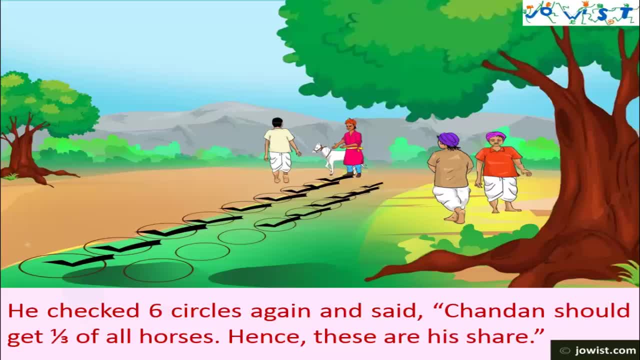 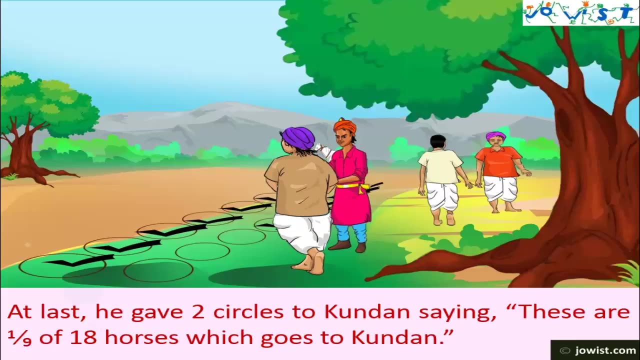 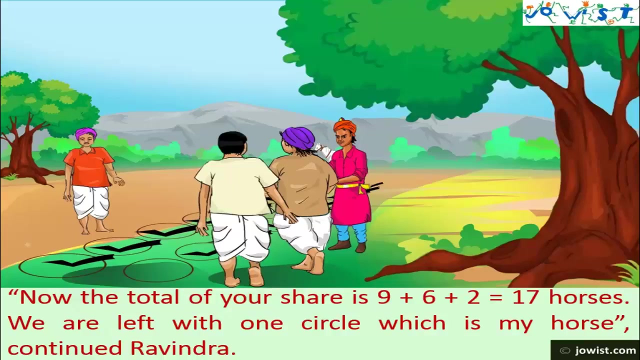 again and said Chandan should get one third of all horses. Hence these are his share. At last he gave two circles to Kundan, saying these are one ninth of eighteen horses which goes to Kundan. Now the total of your share is nine plus six plus two. 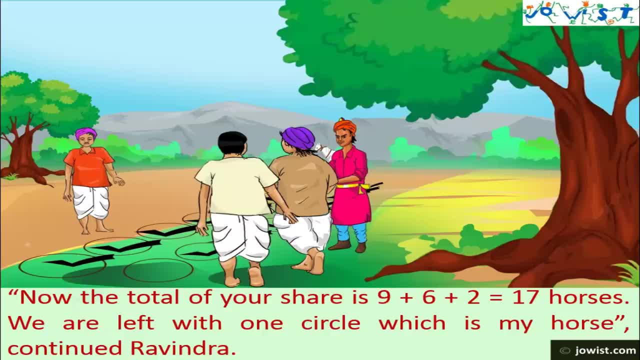 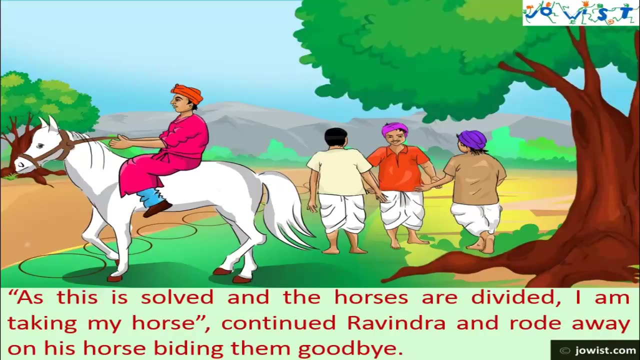 That is seventeen horses. We are left with one circle, which is my horse, continued Ravindra. As this is solved and the horses are divided, I am taking my horse, continued Ravindra, and rode away on his horse, bidding them goodbye. 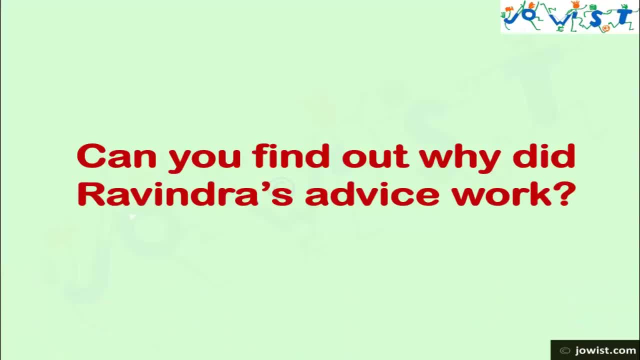 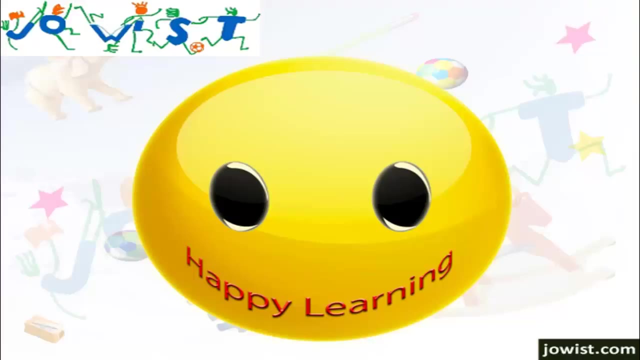 Now you have heard the story how Ravindra's advice worked. Can you find why did Ravindra's advice work? Happy Learning.